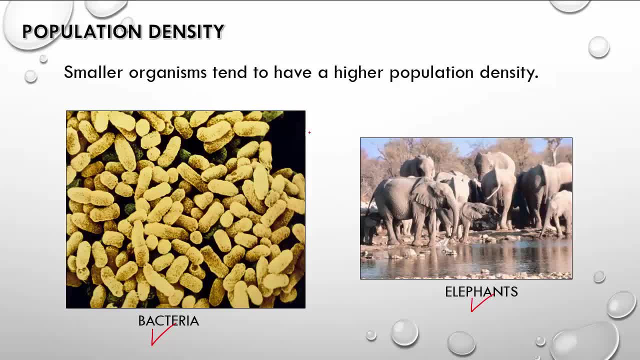 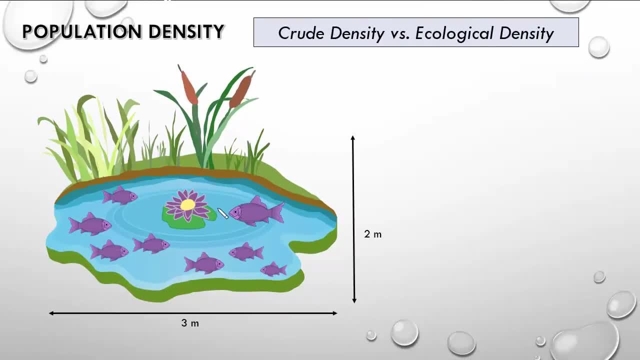 There's a high population density here, but there's much more of a higher population density in the bacteria than in the elephants themselves. So now we have a pond with a number of fish and we want to calculate the population density. So population density equals the number of organisms divided by the space. 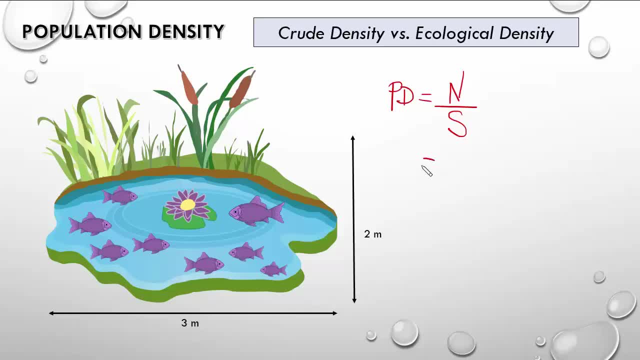 Or divided by the volume or the area. So in this case we have 1,, 2,, 3,, 4,, 5,, 6,, 7,, 8 purple fishes or fish in this pond here. So we're going to have 8 divided by the space or the area. 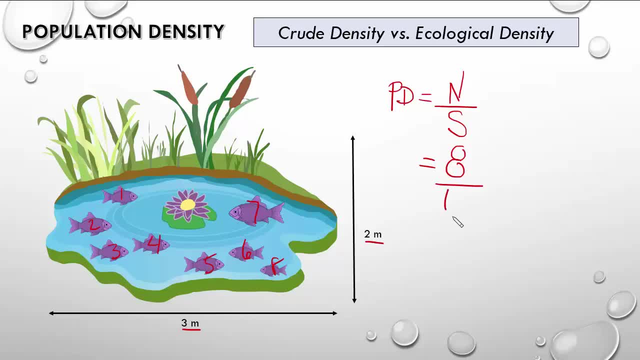 So we've got 3 meters by 2 meters, so that's going to be 6 meters squared And this is 8 fish, And so when we divide these out we're going to get an approximate population density of 1.3 fish per meter squared. 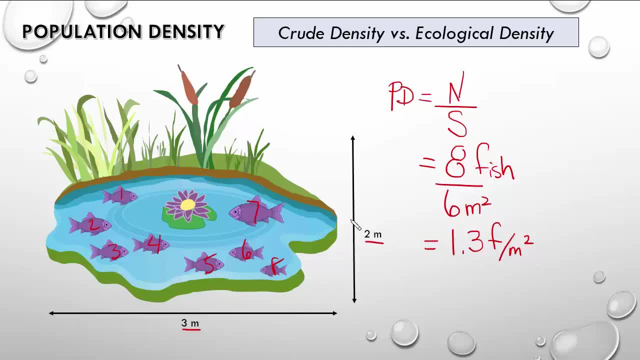 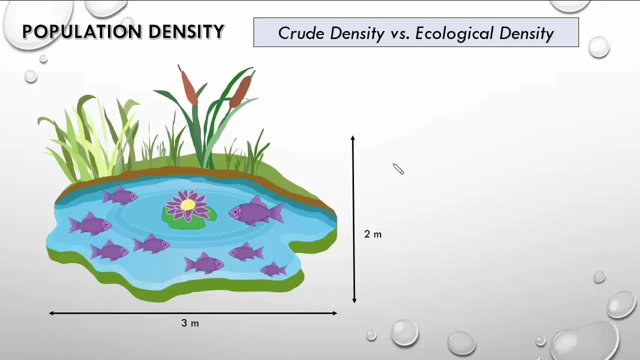 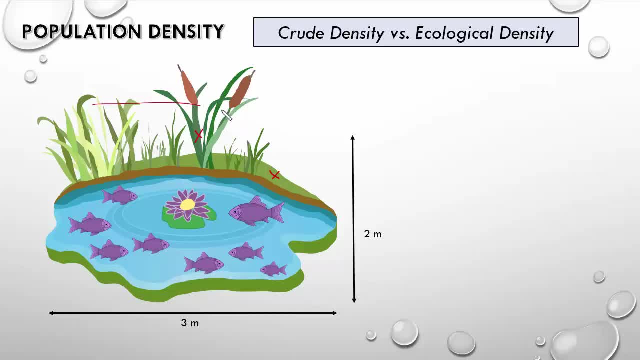 They're not on the plants here, which is all part of the calculation here for the space involved with population density. So the crude density was what we just calculated. So the crude density was what we just calculated. ecological density is the area that's actually used by the organism, so of 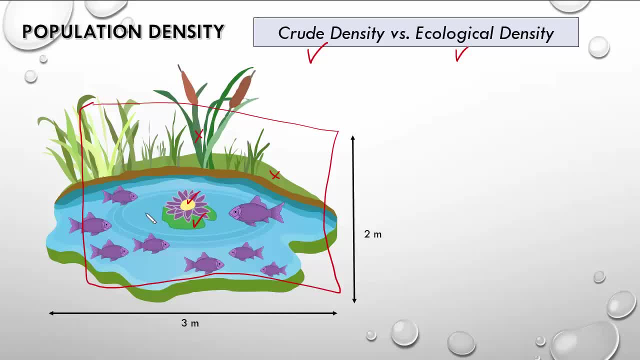 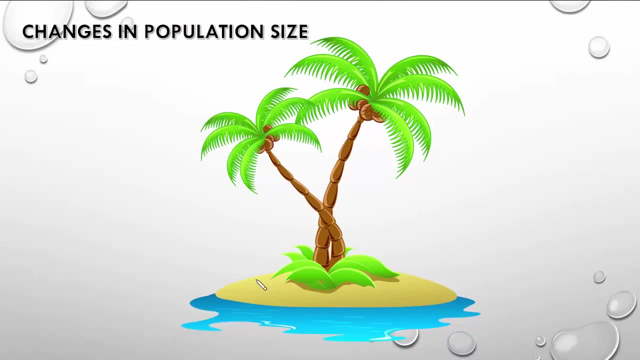 course. then you know they're not on the lily pad here on the flower, they're just in the water. so the ecological density is going to be smaller than the crude density. so populations, of course, do not remain static. they change over time and the reasons that they change. if we look at this little island here is: imagine: 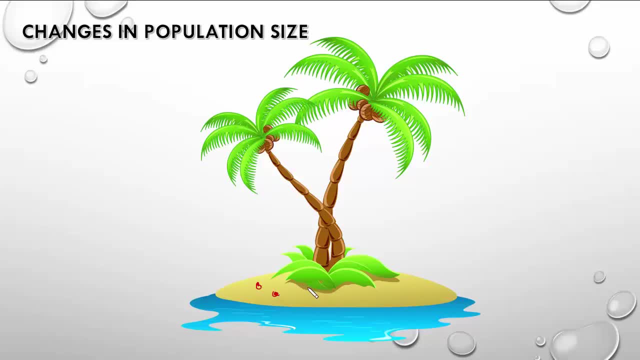 that we've got an organism over here, we've got an organism over there and these guys reproduce and there are more organisms on this little island here and that would represent the births. so as individuals are born, they are going to increase the population size. sadly, some of these organisms are going to die, so 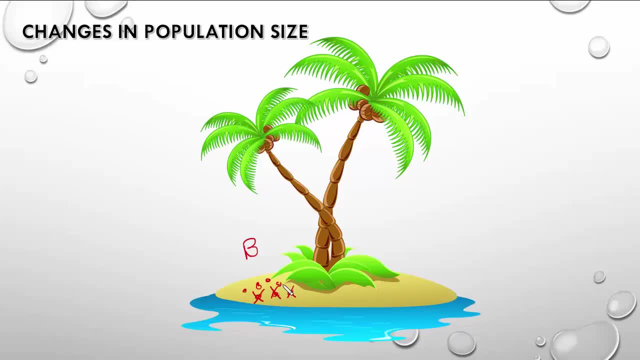 let's say, this guy goes and this guy goes, and that guy goes and that's going to change the population size as well. so now we're talking about deaths. so we have births that influence population size, we have deaths that influence population size, and then along they come swimming through the water. 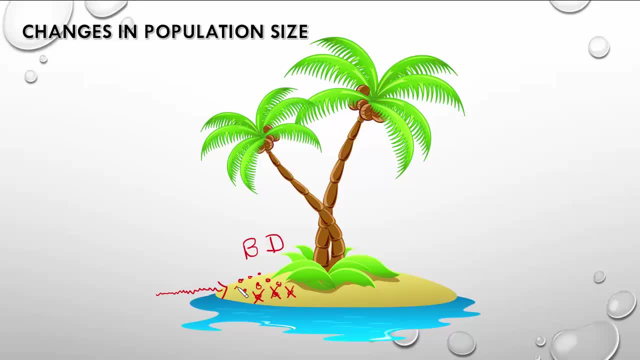 landing on the island and they decided, hey, I like this island and so they've joined here. so we have some immigration to the island and that's going to increase the population size. and then this one says I'm out of here. and this one says, okay, I'll join you, and they leave, and so we have emigration as well. 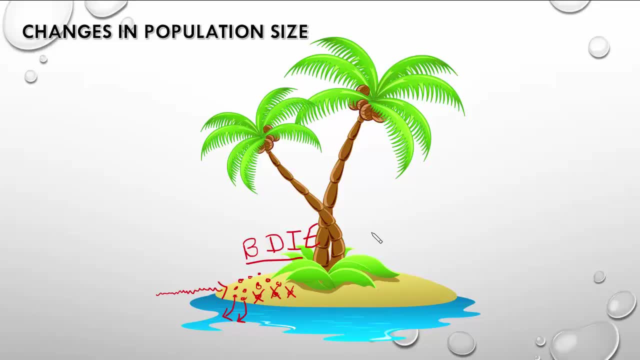 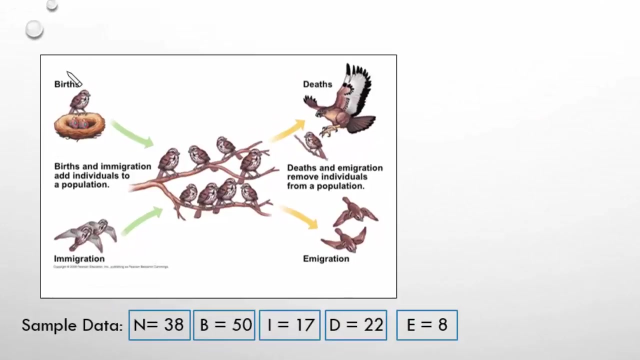 so we have these factors that influence the population size: birth, death, immigration and immigration- all causing changes in the original population number or the population size. so let's have a look at an actual calculation of changes in population size. here we can see that for these birds, births occur. 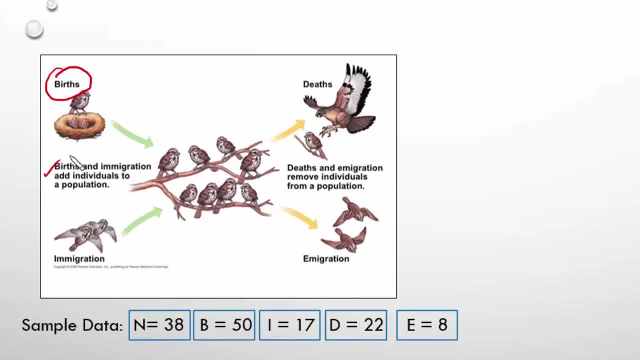 and that's going to increase or add to an entrance point. so if I exit the island here we can see that births are required and that's going to increase or add to a population size. deaths occur and that could be due to predation or just natural causes or disease or 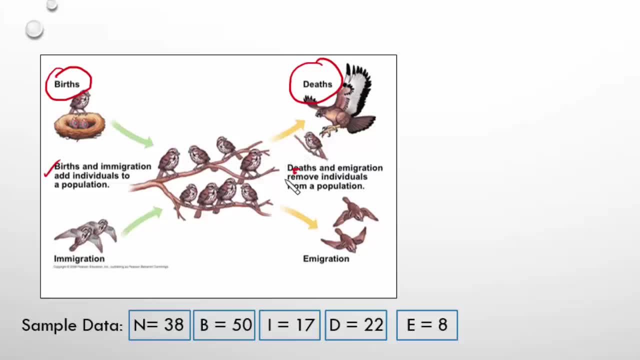 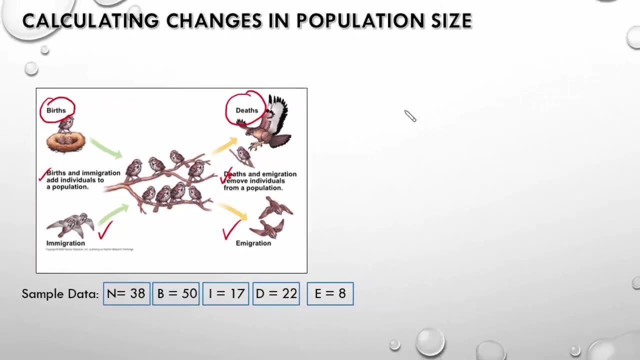 whatever, and that's going to remove individuals from the, from the population. we have immigration adding to the population and emigration as they leave. so let's imagine we have this problem here, all right, and let's calculate the change in the population size. so let's call this: 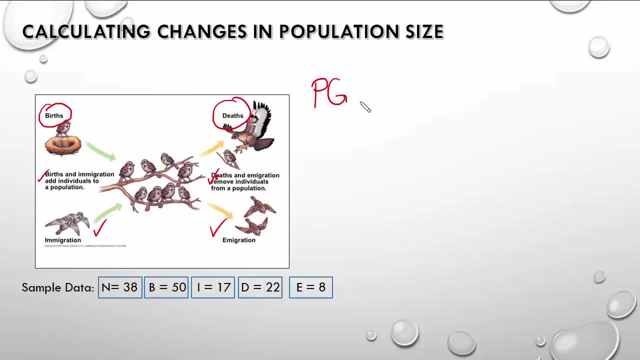 population growth and, of course, growth can be negative or positive. usually when somebody's growing right, we think they're getting tall or whatever. we don't think of them as getting short. we always think of it as a positive thing. but population growth or population change can be either positive or negative. so what we're going to get is population growth or 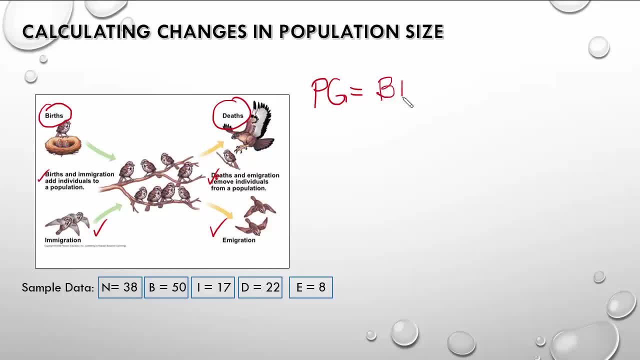 change is equal to births plus immigration. all right, those two things are going to increase the population size minus deaths and emigration, and those are going to decrease the population size. this is going to be divided by the original number of the population and we're going to multiply this. 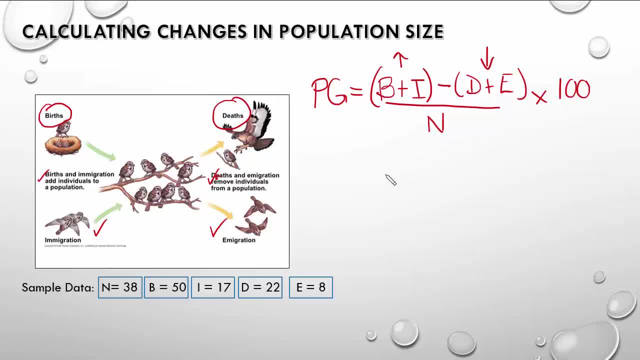 by 100, because we'll get a percent or a decimal or something like that. okay, so the number of births in this example is 50 plus the immigration is 17. so we've got that minus the deaths, which are 22, and the emigration, which is 8. we're going to multiply this by 100. 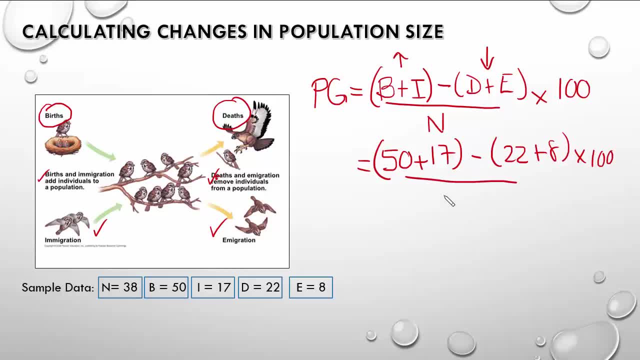 and we're going to divide it all by the original population of 38. so when we do the math, we're going to come up with 67 individuals that have been added to the population, minus 30 individuals that have been removed from the population, divided by our 38 times 100. 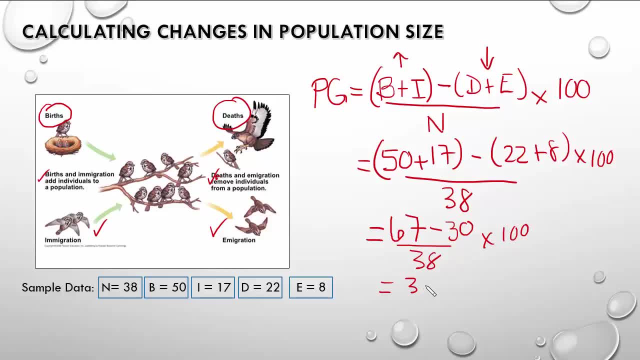 so we're going to end up with 37 individuals, whereas we had 38 in the population at first, times 100. so we're going to get around 0.97 and when we multiply it we're going to get around 97 percent. so what we can see is that the population has declined. 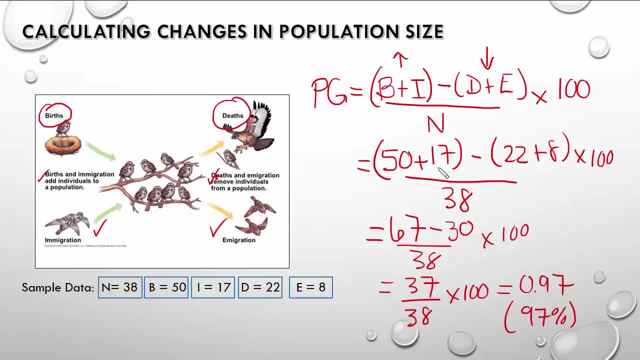 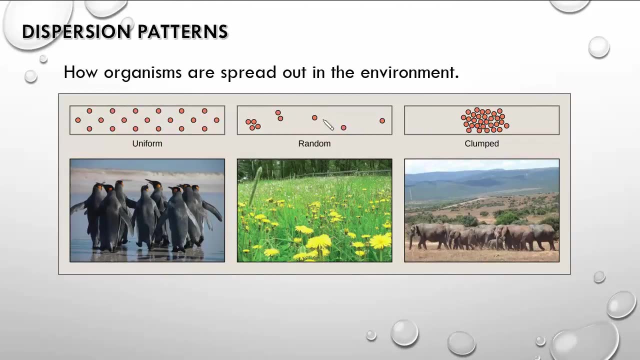 by about 3%. due to the births and immigration, deaths and immigration, the population has declined, so that is a change in the population size right there now. another concept that we need to deal with is that of dispersion patterns, and dispersion patterns are how organisms are spread out in the, in the 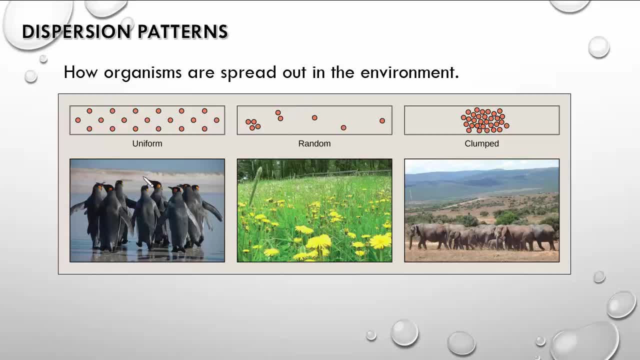 environment, and here we can see some penguins that are exhibiting something called uniform dispersion. we've got some grass and flowers that are random and we've got some elephants that are clumped. so a uniform dispersion is just as it sounds, where the organisms are very spread out in very balanced fashion. 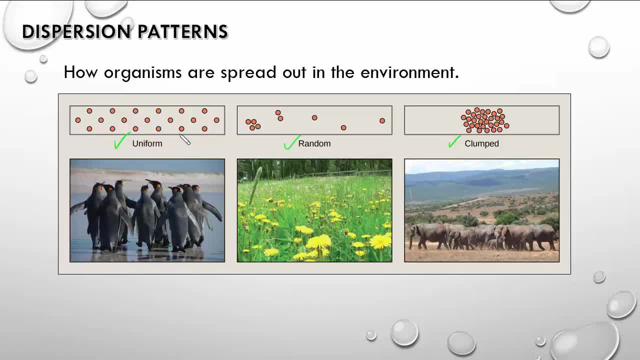 very uniformly, very organized, all right, and this is not a very common pattern. it is exhibited by some organisms. this does not. by the way, this image, which does go with uniform, does not look like this is uniform dispersion. this actually looks more like it's clumped dispersion. all right, but 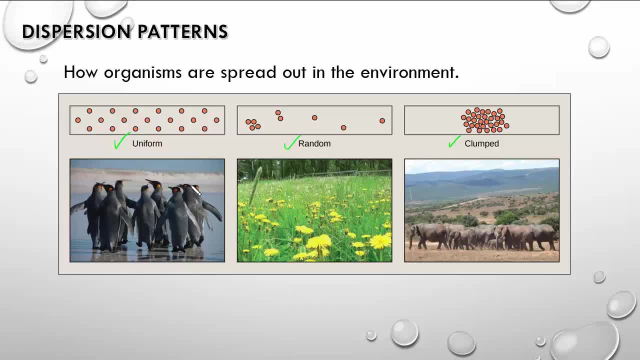 these are the images that went with this particular graphic and is trying to illustrate it. I don't think it's the greatest one now that I have a close look at it, but this can occur when organisms are going through their mating season, like a bunch of birds on an island or something, and they need a 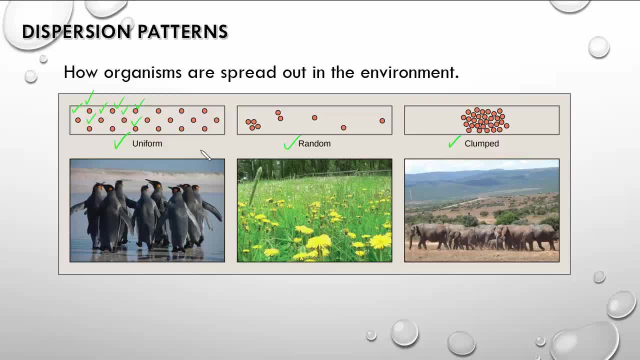 particular amount of room- don't worry, I'm not gonna put a checkmark beside everyone- and they need a certain amount of room between the, the breeding couples, so they'll spread out uniformly. uniform dispersion is also seen when, say, farmers plant their fields and they've, you know, they put down the rows of corn. 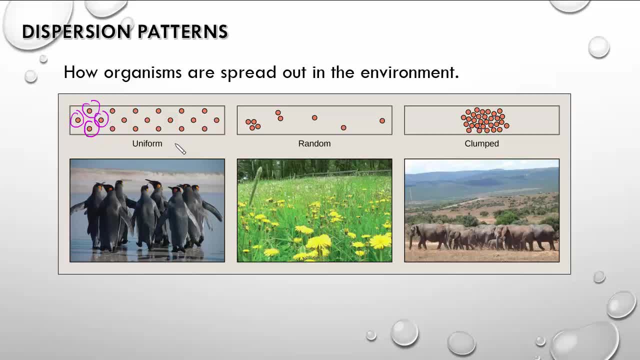 or wheat or whatever, and we get this uniform dispersion. random dispersion is what you would tend to expect with things like trees, with with grass, with flowers, that you know wherever the seeds land and take root, that's where they grow. so you get this very randomized type of dispersion. now, of course, there are interactions between 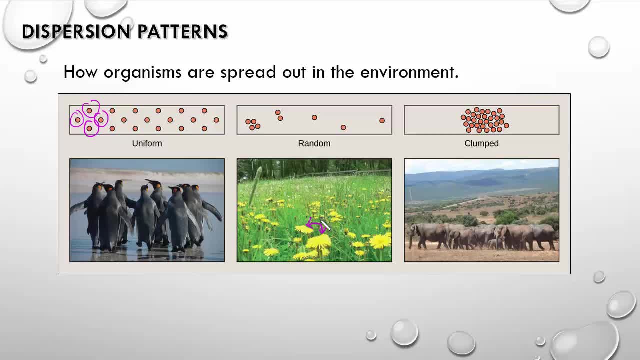 these plants all right, and between the grasses they release chemicals that sort of keep other plants away from them a little bit so that they can have access to the nutrients below the soil. there is actually some interaction between these organisms, and so there it's not exactly random. 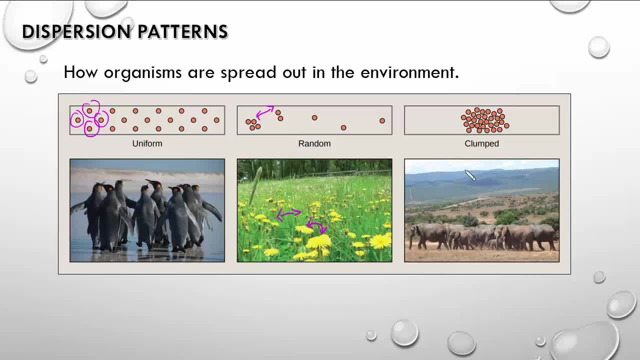 but it's a good approximation, so we're just going to leave it at that. many organisms exhibit clumped dispersion patterns, like this group of elephants that are on the go together, or organisms that hunt together or feed together for protection, for providing for the offspring, whatever schools of fish flocks. 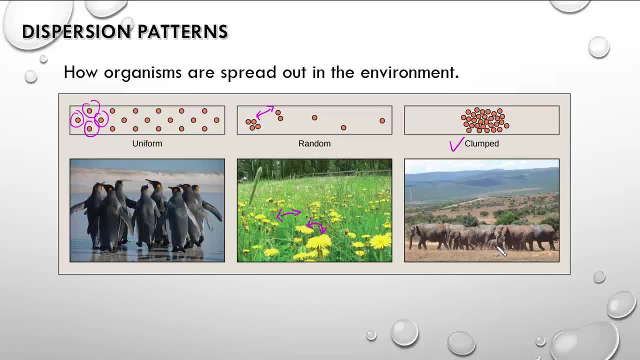 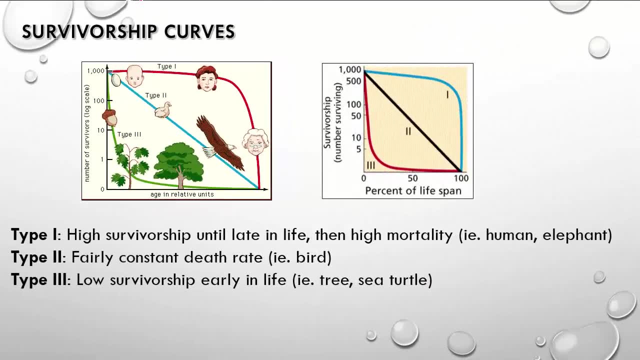 of birds, all of that thing. ok. so uniform, random and clumped dispersion patterns are the ones that we are concerned with, with all right on to survivorship curves. now survivorship curves come in three types. there is type 1, type 2 and type 3, and when we look, let's have a look at 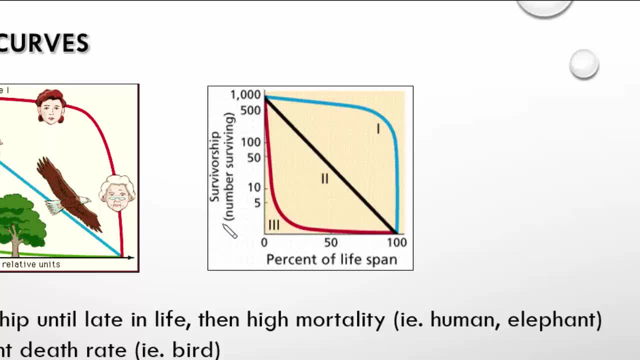 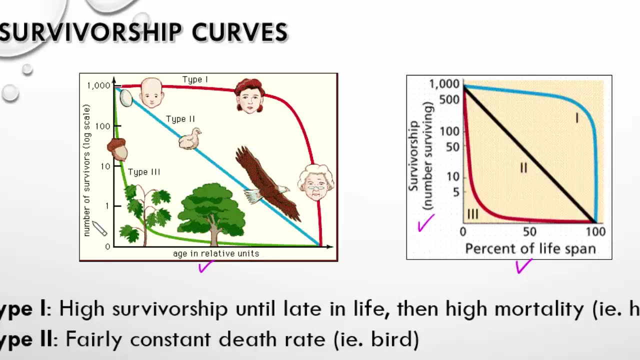 the axis. here we're looking at the survivorship, or the number of individuals that are surviving over time, the percent of their lifespan, or over here, the agent relative units. all right, so this is the number of organisms here on the Y over their lifetime, and there are three types of curves. all right now. 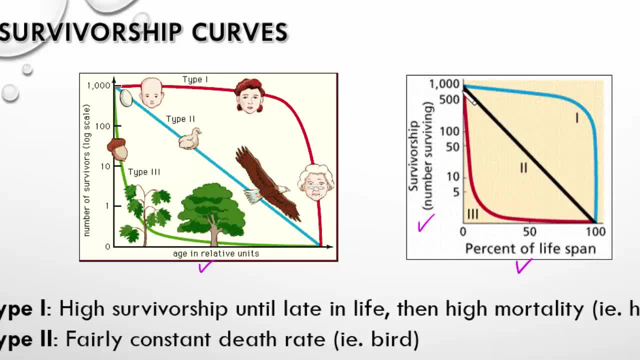 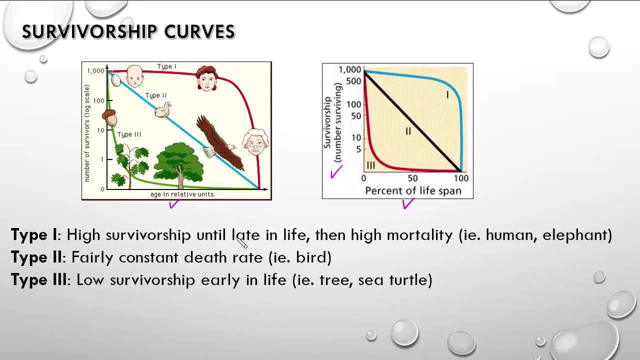 don't worry about the fact that the colors are different here. all right, but you can see type 1, type 2 and type 3 and they look the same in both of the graphics. type 1 survivorship curve is illustrating high survivorship until late in life. 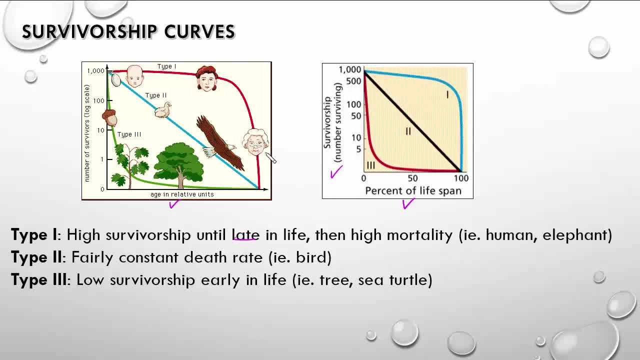 and then there's a high mortality. and this is the typical pattern that that humans go through. that elephants stuff like where the individuals are born and many of them survive at birth and they live a long life and then later in life there is high mortality. so there's a good long life here and then, as they get, 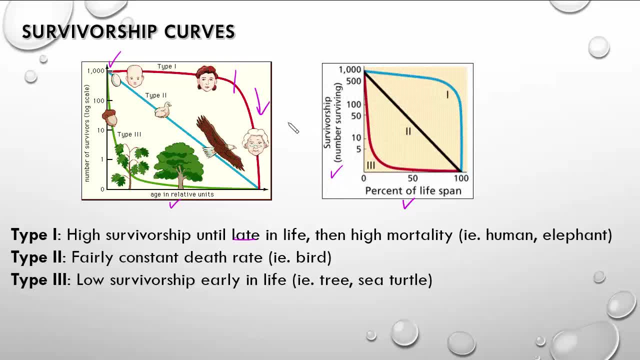 to a certain age, then they die off rapidly. all right, elephants do this, humans do this, stuff like that. let's contrast that with the type 3 survivorship, which is somewhat different. this is low survivorship early in life. but if they survive that period they do tend to live. 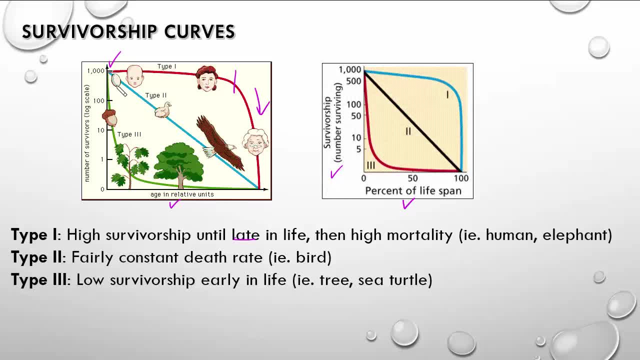 a long life. so, for example, trees and stuff- just imagine how many seeds are released, how much pollen is released. the survivorship is very low for these organisms early on, so you see them dropping off early in their life cycle. many of them don't make it, and then those that do, though, tend to live a nice 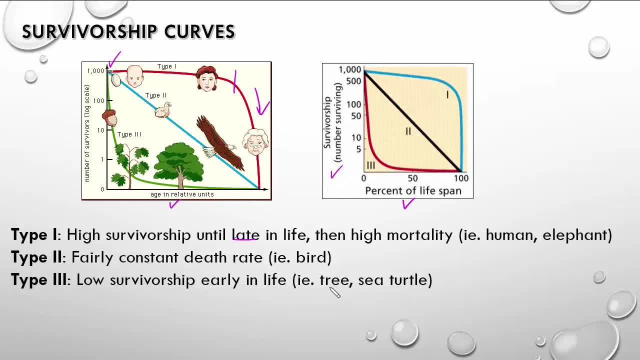 long time. so think of trees in the forest right and trees in the rainforest. some of them are hundreds of years old. if they took root and survived, they can live a really long time. same thing with sea turtles. all right, they. there's lots of offsprings and there's a lot of offsprings and there's a lot of. 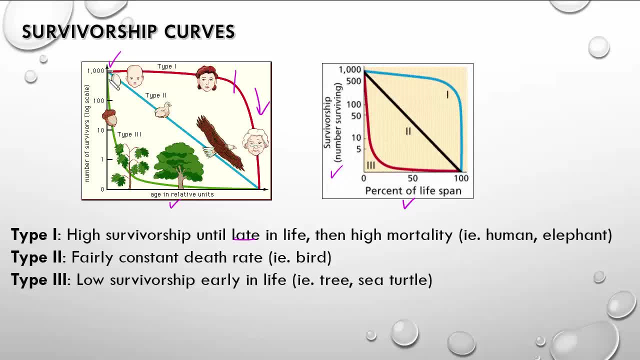 offspring, but the chance of them surviving is very low. but if they do survive, they live a long time. they become old and wise like grandma. here, all right right in the middle, we have a fairly constant death rate. so for example, for birds there are squirrels. the chance of survival is it's hit or miss and it's 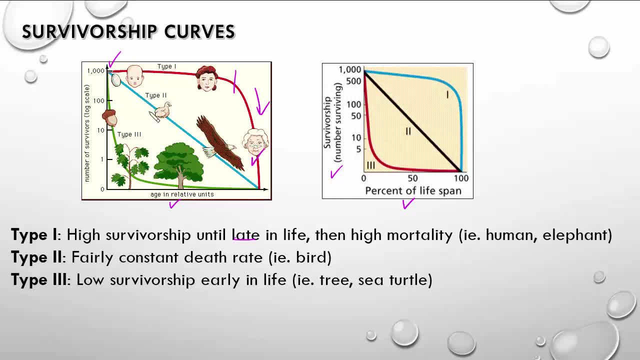 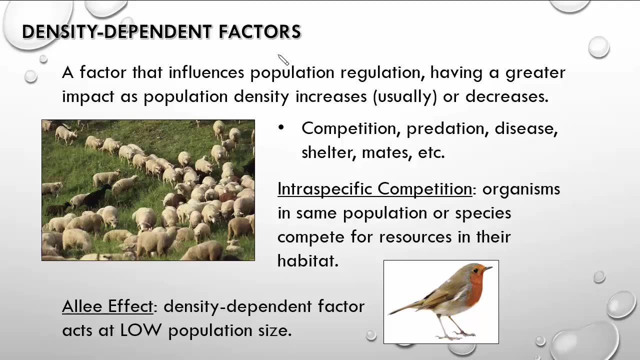 pretty constant all throughout their lifetime. so it's just this linear relationship, all right, all right. so survivorship curves- type 1 curve, type 2 curve and type 3 curve. let's talk about density dependent and density independent factors in ecology, a factor that influences population regulation having a greater impact as population. 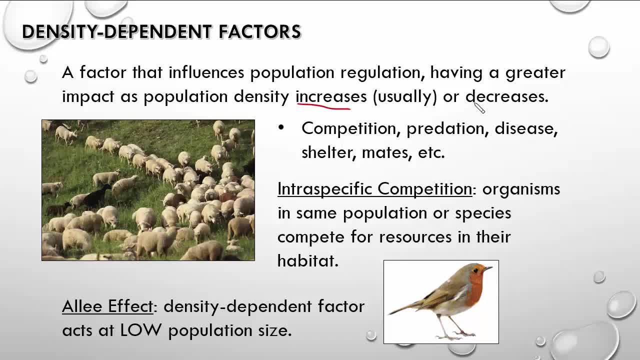 density increases usually, or decreases usually. we think of increases as things that are going to be affected by density dependent factors. usually we think of increases as things that are going to be affected by density dependent factors. examples of density dependent factors are competition, so here we have an image of some. 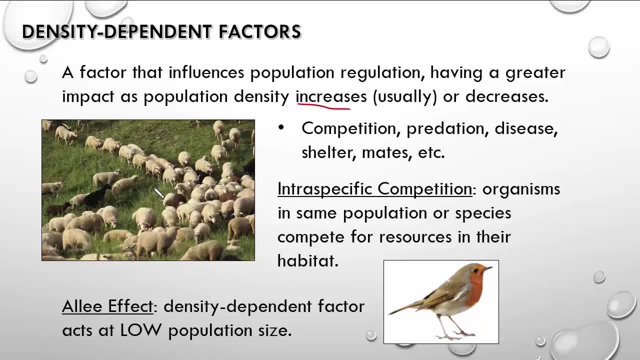 cattle, herds of animals, anyhow on the plains, in the grassland, where they may be, and they are competing for resources, they're competing for food, they are competing for shelter and for mates, and all of that is a density dependent factor. i mean it depends on how many of 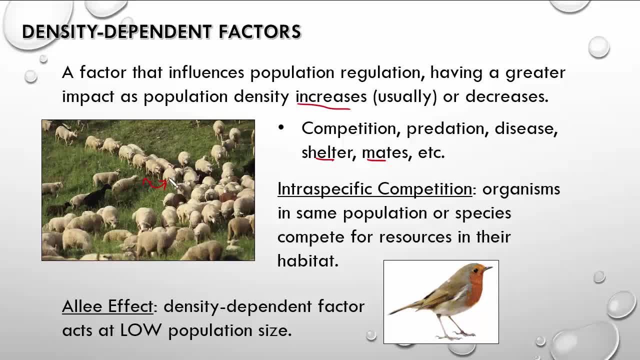 them and then then גם t testi này characteristics. sau đó đốita vraag các là các khác. there are high density dependent factors for the loss of diversity. Now, in this conceptal culture, we now have what is a, And the more that there are, the more interactions there is and the less shelter there's going. 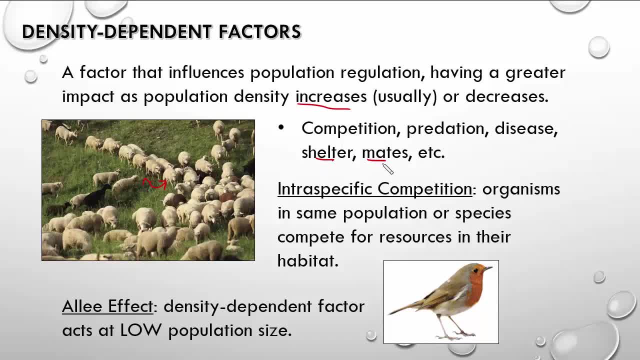 to be available or the less mates there are going to be available. Predation can be sort of a density dependent factor, because here comes the predator- I know that's not a predator, but just imagine- And there's a whole bunch of them. 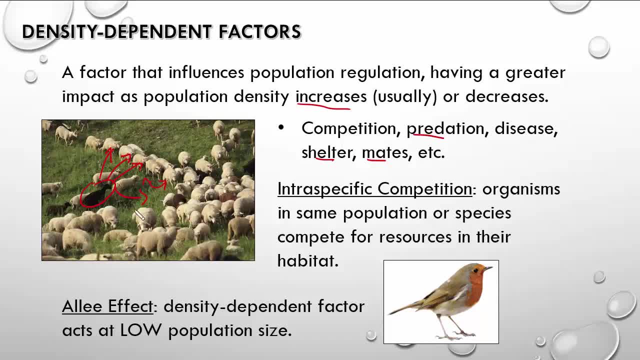 Pick off this one or this one or this one, that kind of thing. So as the number or the population size increases, as the population density increases, this factor becomes more important. There's more of them to be attacked. Disease is often also found in high population numbers, because this guy gets sick there. 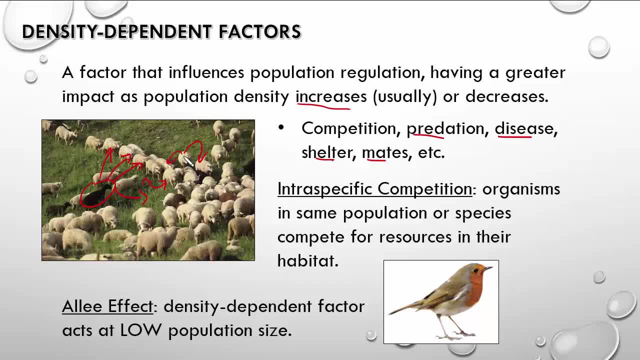 and can pass it to this one and to this one and to this one because it's in such close proximity to these ones. So the increased population density, It actually lends itself to the transmission of disease. So this concept of interest, specific competition, is what I was talking about before. 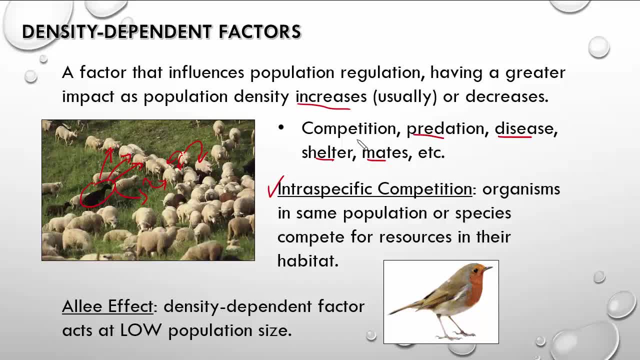 As a density dependent factor. the more the population density increases, organisms in the same population or species will compete for resources in their habitat. So on the grassland they are competing against each other. It's not like a lion attacking, You know, a gazelle or something like that: throughout the same species competing for 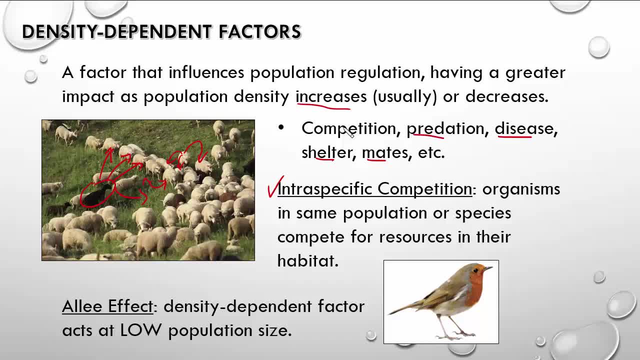 the same thing. So again it's competing for shelter, or for mates or for food, all of the same resources. So this is dense. These are density dependent factors. They depend on the density of the population and they can regulate or limit the population. 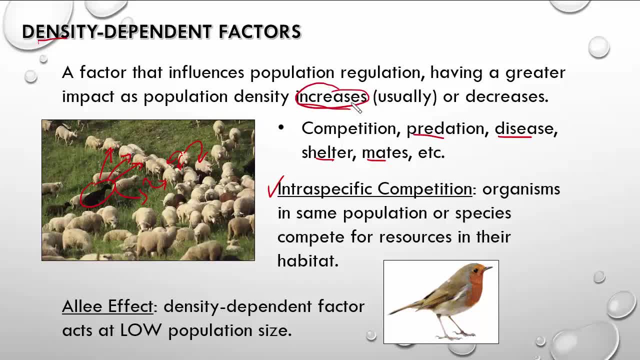 Now we've been talking about Increases in population density. Well, there's something called the alley effect, which is where a density dependent factor acts at low population size, And I give the example of this bird here. Imagine that, instead of there being a lot of birds and this little guy or gal is competing. 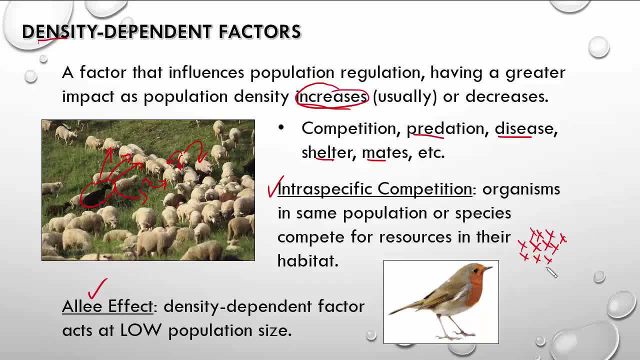 for food and mates and shelter and all of that stuff. Imagine if there are very few of these birds. Now The odds that it will get to mate are actually quite low, despite the fact that there might be lots of worms or lots of seeds and space and all of that stuff. 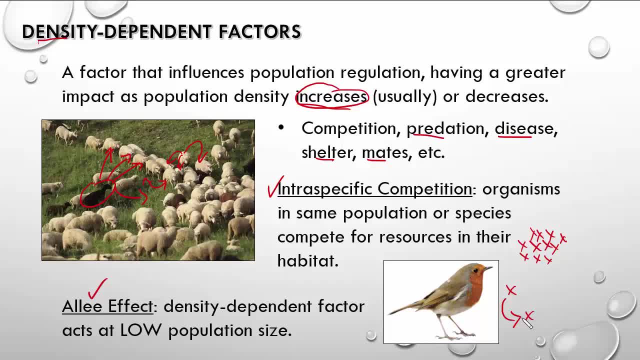 If the population gets too low, then they can't mate properly. And even if they could mate, there might be some inbreeding going on, where you know they're mating with each other and with siblings and stuff like that, So they're not going to have a healthy population. 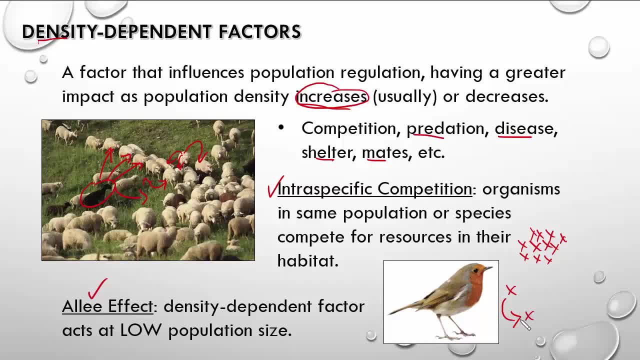 This is called the alley effect, which is somewhat contrary to what you might Think When you think of an increase in population density causing all these things. right, It's obvious we're going to have to compete for this stuff. Well, if the numbers are too low, the alley effect kicks in, which is a density dependent. 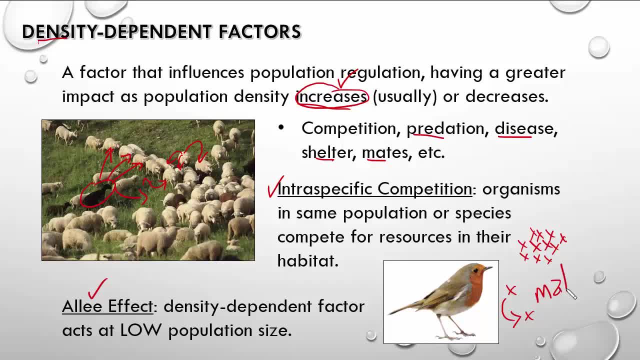 factor, with respect, for the most part, to mating. You can think of it that way: If you have a low population, mating is now a density dependent factor. I mean it depends on the density of individuals to have mating. The density happens to be low. 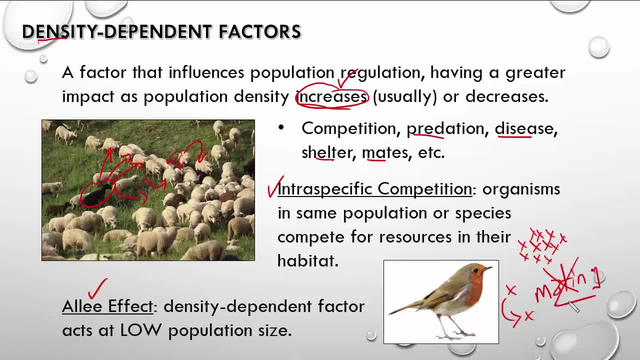 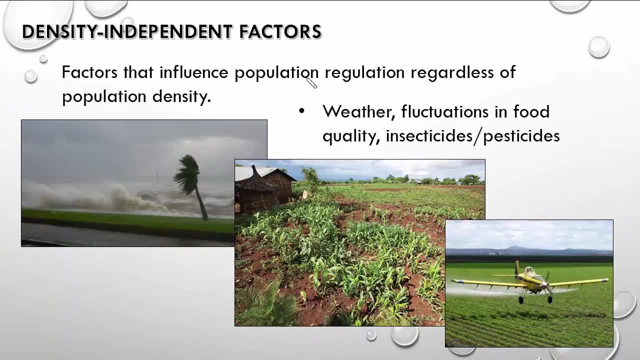 So not a lot of mating going on, and this this can lead to the extinction of a species. Density. independent factors are factors that influence a population or the population density, regardless of the actual population density itself. All right, So they influence the population, but regardless of what the population density is. 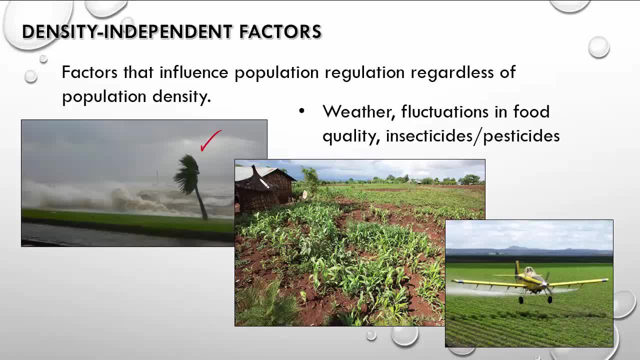 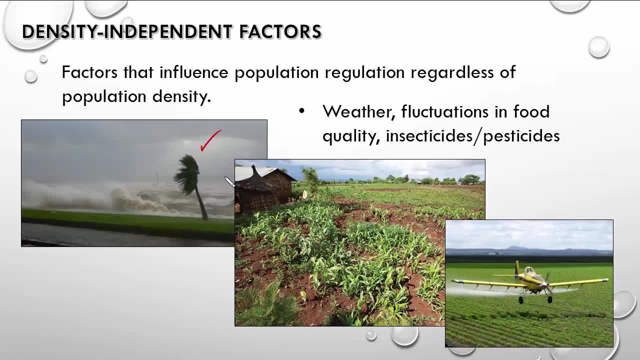 uh, uh, uh, uh uh. Um, humid conditions, droughts, all of those things that don't specifically depend on how many individuals they are there are. uh, it just comes along and it, and it has an, it has an effect. 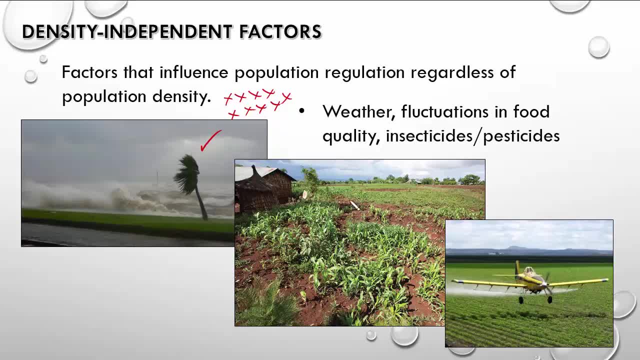 This would be a density independent factor. Um, if you look at this image here, I've tried to find one where the crops you know kind of look like they're not that healthy. Um, it doesn't matter how many individuals are out here grazing. 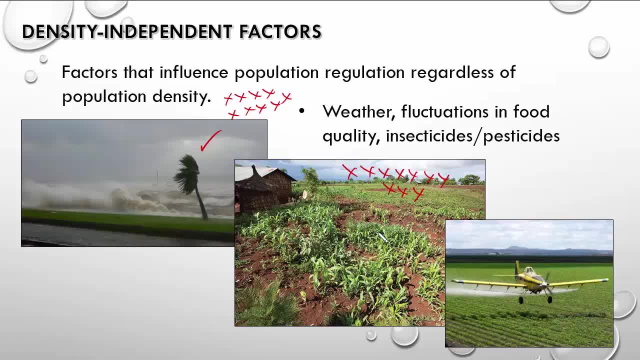 All right, Um, If the crops are not healthy, then they're not getting good nutrition, and that can influence the population size, uh, that can influence whether or not they mate or how they produce all the chemicals they need, The hormones, the gametes, uh, the. the nutritional quality is very important and that's a density. 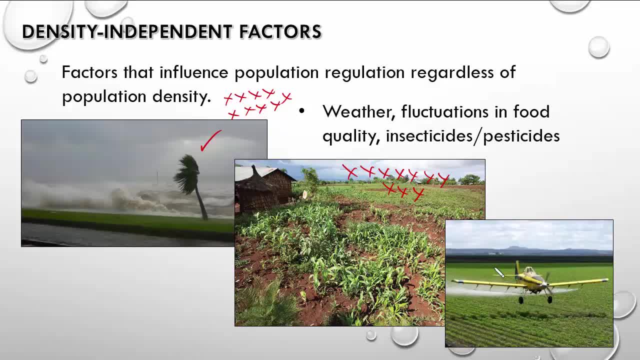 independent factor: the food quality And also humans? um indirectly affect the population density when we spray insecticides or pesticides? Um sure, that is, you know, affecting organisms in the grass here or in the crop, killing them or whatever. Um, but it's not dependent so much on their numbers influencing each other. 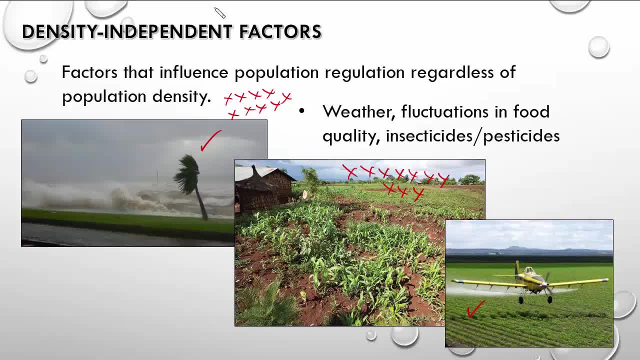 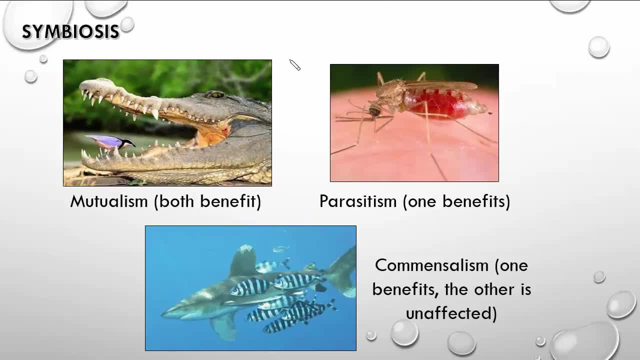 This is something that we've done, and so it's considered a density independent factor. Now, the last concept that I want to talk about in this particular video is one of symbiosis, and you've probably seen this before: Sim referring to same bio for life. 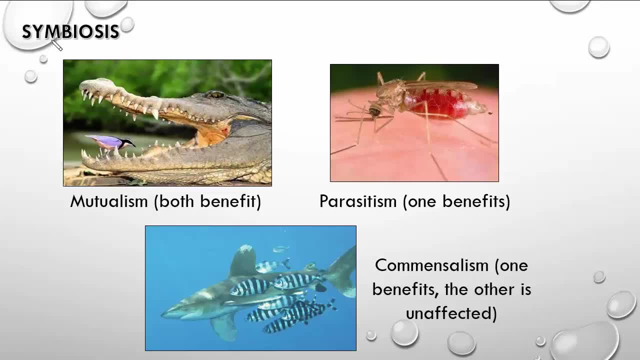 So same life. So, uh, individuals living together, usually in physical proximity, um having an effect on the other one's life, And there are three types. We've got mutualism, parasitism and commensalism. 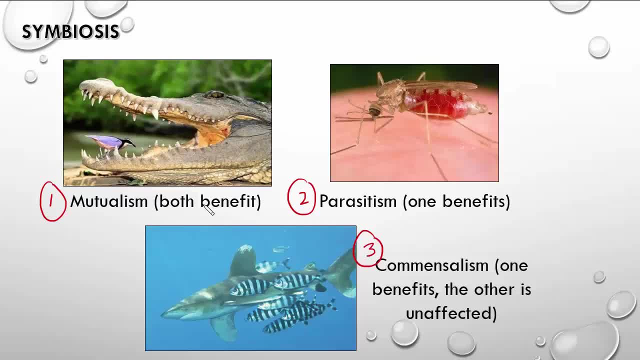 In mutualism, both organisms will have some form of benefit. So here we see a bird in the crocodile's mouth. The bird is feeding on some Debris left in the crocodile's mouth, So so the bird is going to gain here. 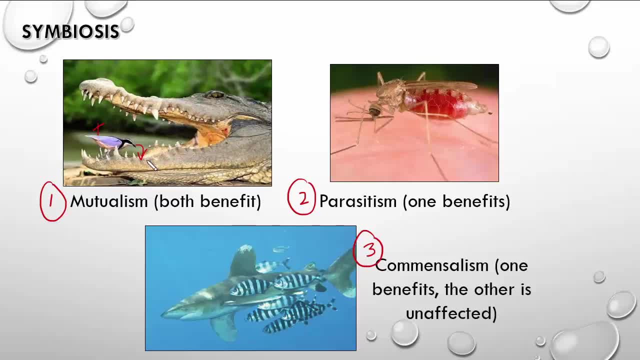 The crocodile gains by having his teeth cleaned out. Maybe there's some microbial life living in there that would be harmful for the for the crocodile. So the crocodile also gains. So it's a mutual relationship. This is called symbiosis. 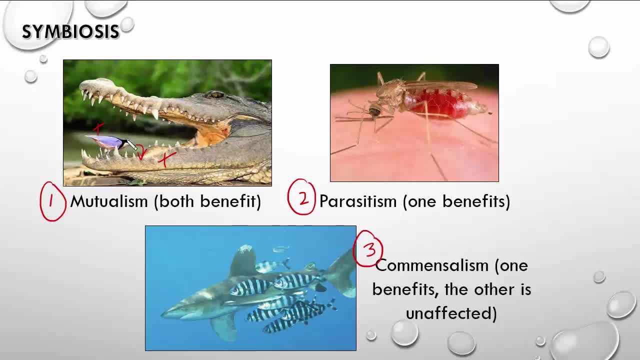 And there are plenty of examples in nature where organisms live together, work together, Um, and they both benefit, And this is a form of symbiosis called mutualism. Parasitism is probably quite familiar to you- dealing with parasites. In this case, one benefits and one is harmed, or one. 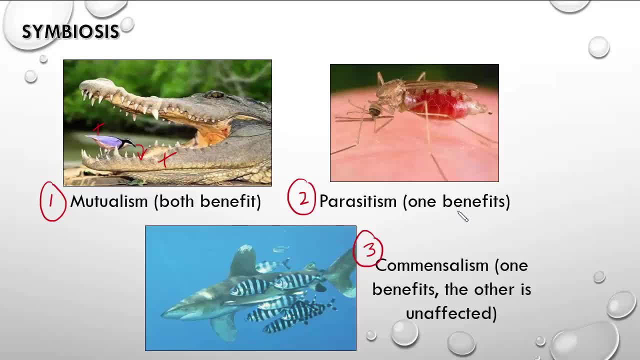 Yeah, One. It's not that one doesn't benefit, is that one is actually harmed? Here we see the malaria carrying mosquito on some human skin, And so the the mosquito is feeding, Of course, taking in the blood, getting the nourishment that it needs. 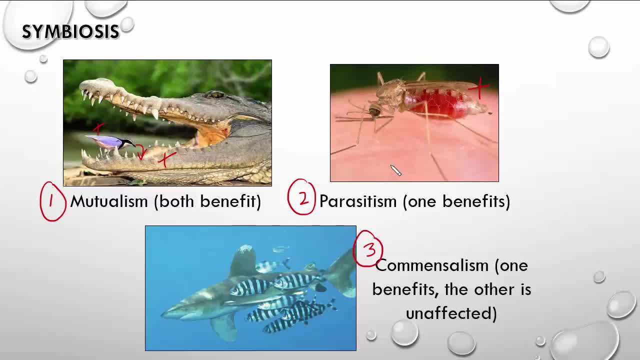 So the mosquito is gaining, but the human, the host in this case- is losing, in that it's losing its blood going into the mosquito And then. so that's a bad thing for the host, but it also may be getting some of the malaria. 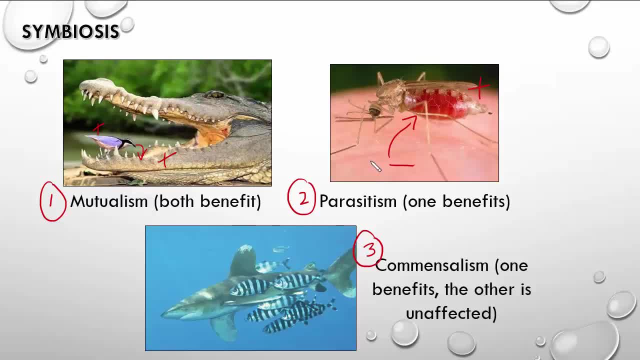 germs, And that, of course, is going to be negative as well. So this is parasitism. Another example is the tapeworm Uh living in an intestine of some organism. the tapeworm gaining the nutrients, the host losing those nutrients.